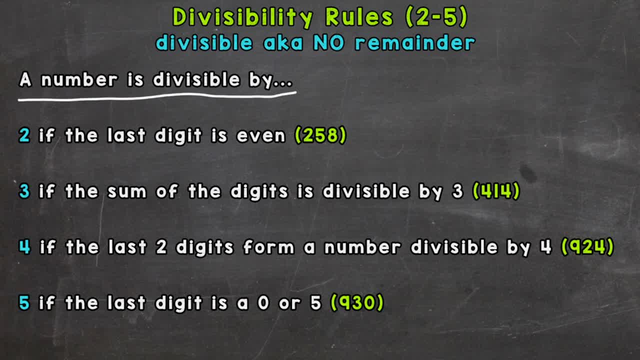 And this is the start of our sentence- for each one of these rules. So a number is divisible by 2 if the last digit is even. So, for example, we have 250.. We have 258. here The last digit is an even number. 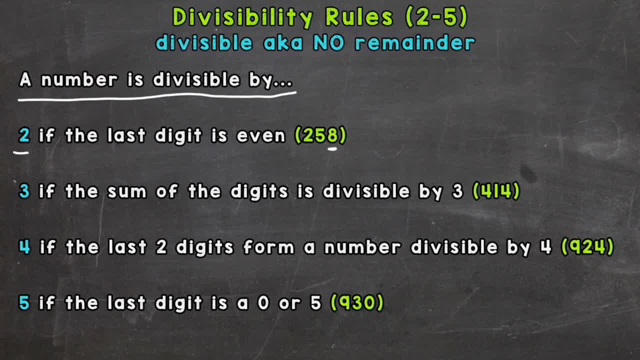 That makes that 258 an even number. Therefore, it's divisible by 2.. We know that we can do 258 divided by 2, and there won't be a remainder. A counterexample would be: let's just do 259.. 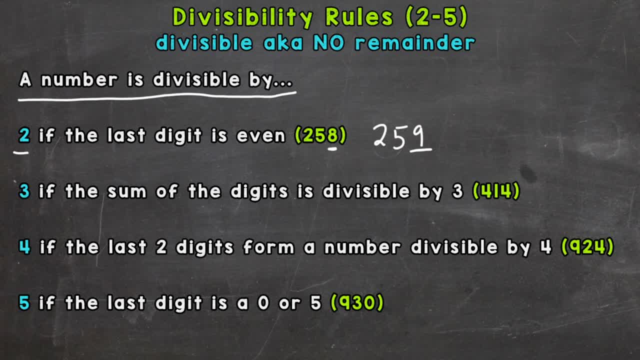 That ends in an odd number. so we automatically know that 259 is not divisible. It's divisible by 2.. Let's go to the next one. A number is divisible by 3 if the sum of the digits is divisible by 3.. 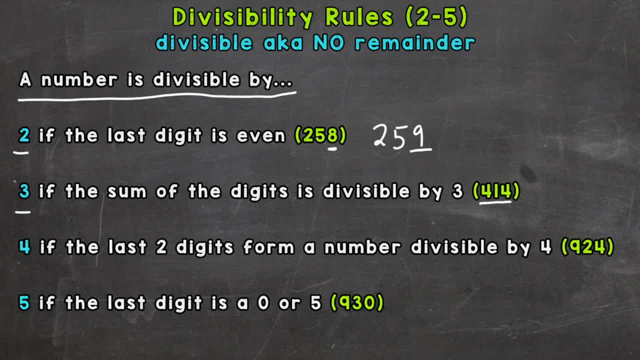 So our example is 414.. So this just means, if we add up all the digits of that number and that's divisible by 3, that whole number will be So 4 plus 1 plus 2.. That's divisible by 3.. 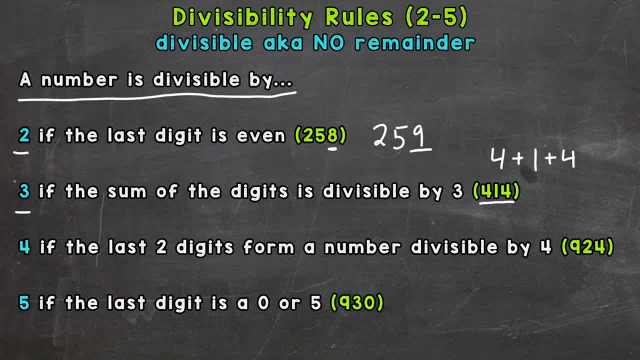 Plus 4.. Well, 4 plus 1 is 5, plus another 4 is 9.. And 9 is divisible by 3.. 9 divided by 3 is 3, without a remainder. So we automatically know that 414 is divisible by 3.. 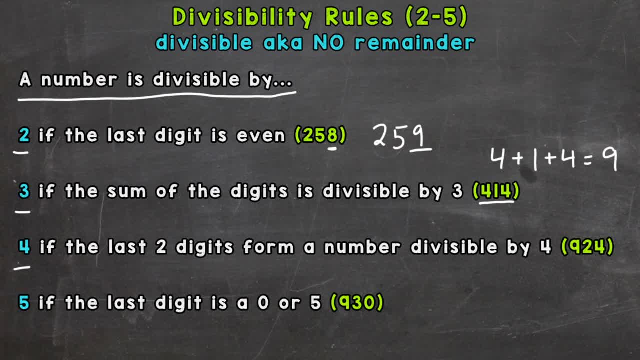 A number is divisible by 4 if the last two digits form a number that is divisible by 3.. So for example here: 924.. The last two digits form a 24. And 24 is divisible by 4.. 24 divided by 4 is 6.. 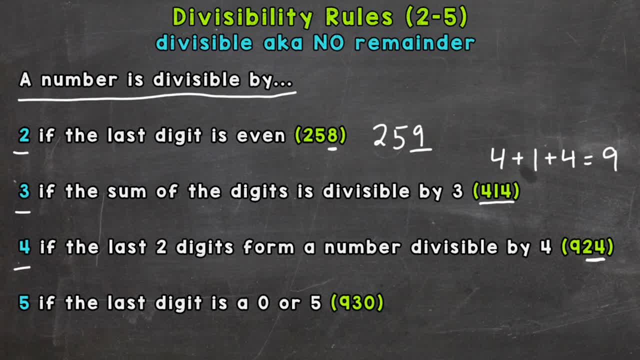 And we don't end up with a remainder. So those last two digits are in fact divisible by 4.. So the whole number will be divisible by 4.. 924 is divisible by 4.. It's divisible by 4. And lastly, 5.. 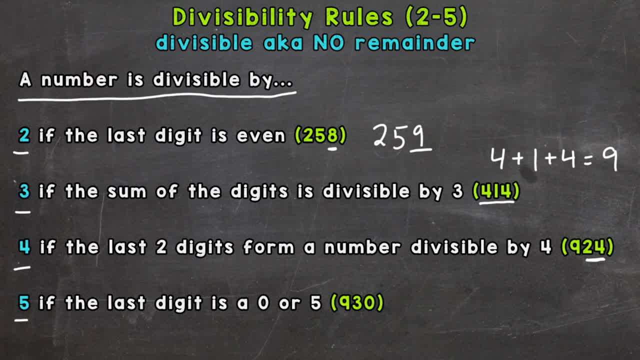 If the last digit is a 0 or a 5.. So simple enough there. If a number ends in a 0 or a 5, it's divisible by 5.. So obviously here, 930 ends in a 0. So it is divisible by 5..